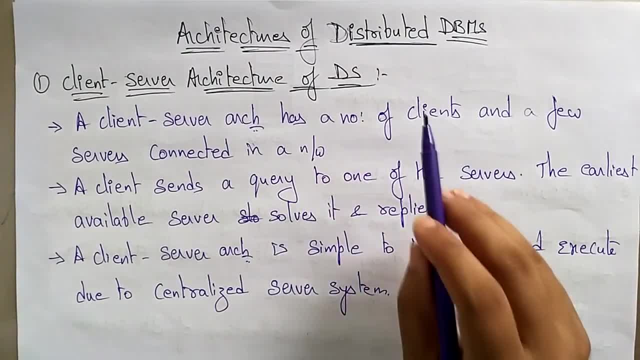 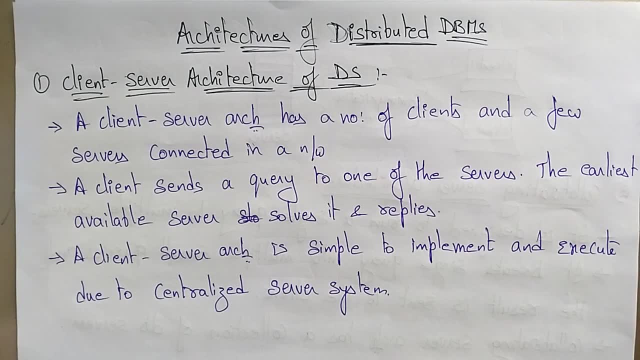 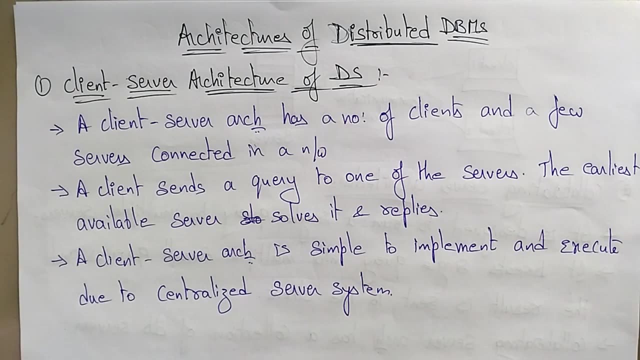 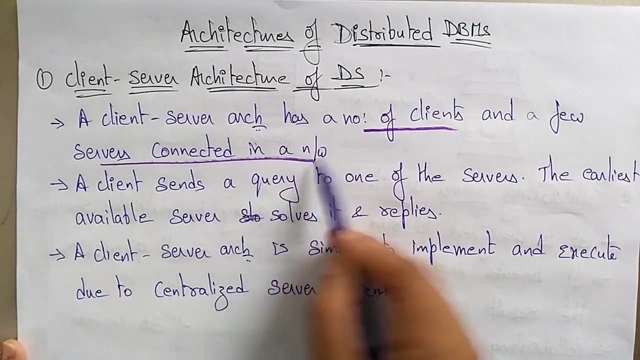 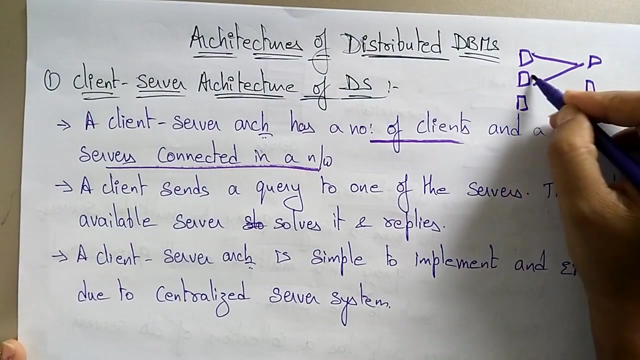 A client-server architecture has a number of. actually, these architectures of distributed database management systems are divided into three types. There are three types of architectures for distributed database management systems. That is the first one is a client-server architecture. Let me explain you: the client-server, A client-server architecture, has a number of clients and a few servers connected in a network. So number of clients are there, okay, and the few servers are connected over a network. 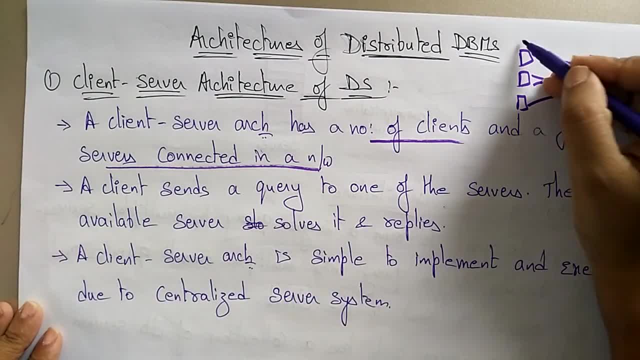 So here, a client sends a query to one of the servers, So this client is sending a query to one of the server. So also, a client sends a query to one of the servers. So here, a client sends a query to one of the servers, So this client is sending a query to one of the servers. 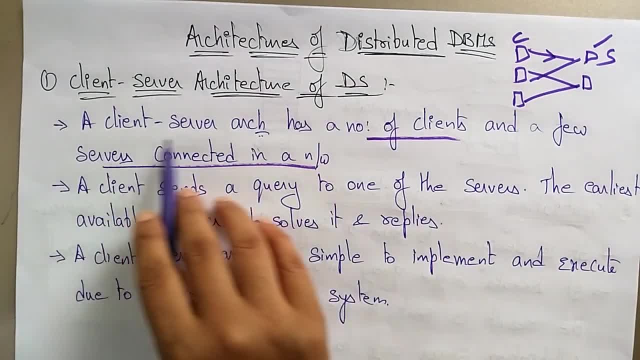 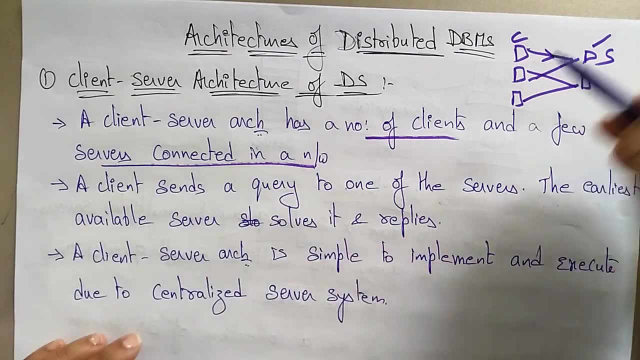 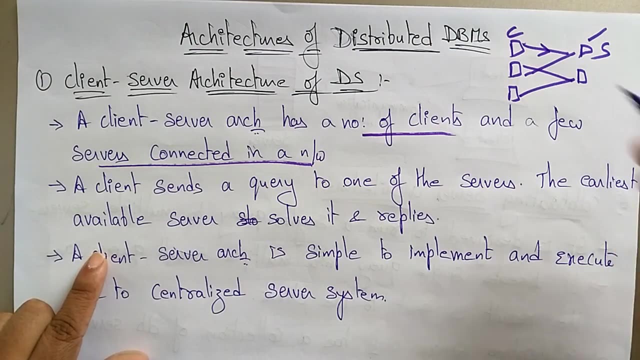 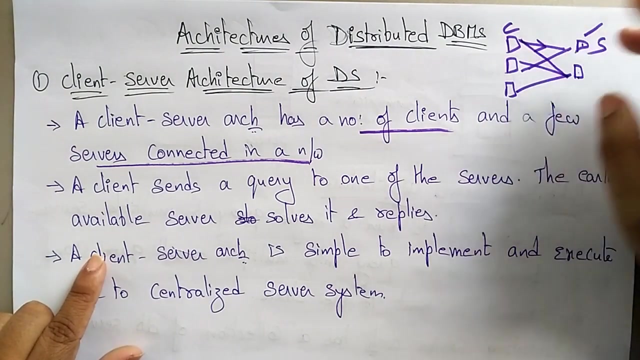 So this client is sending a query Here. the client architecture has number of clients and a few servers connected in a network. A client sends a query to one of the servers. The earliest available server solves its replies. See here: the earliest available servers solves its reply. Either this server or this server. Any one of the server can solve the problem of the client, but the earliest one takes Which server is receiving that client's? 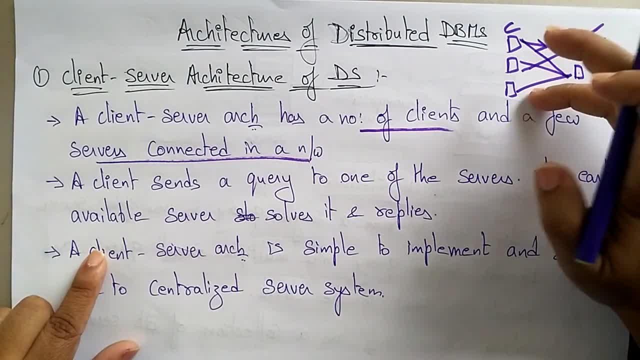 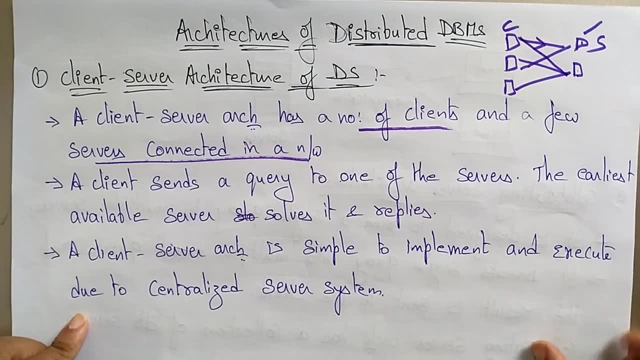 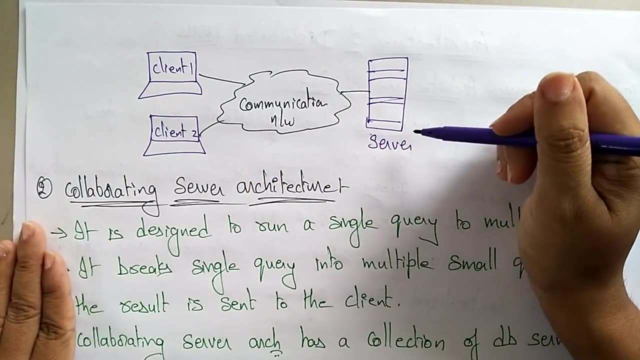 request, that server can able to solve it and it can reply to the client. so the client server architecture is simple to implement and execute due to centralized server system. so see here, this is the client one and the client two and i have taken only one server. if you want, you can take. 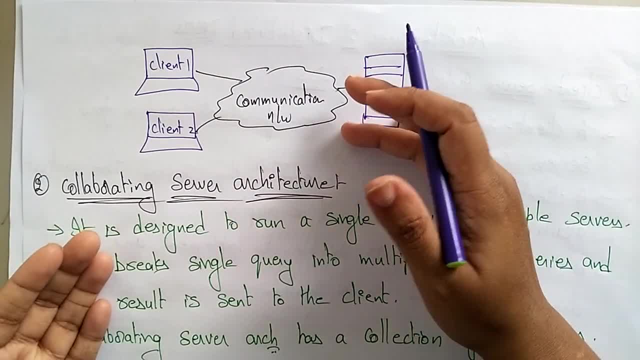 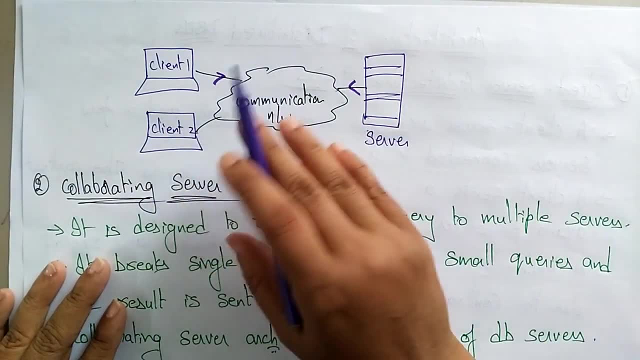 more clients and few servers and communicate it over through a communication channel. so here, whenever the client is asked for request and the server is going to be replied to the client, okay, so this is a client server architecture, but here's the client that's sending the information. 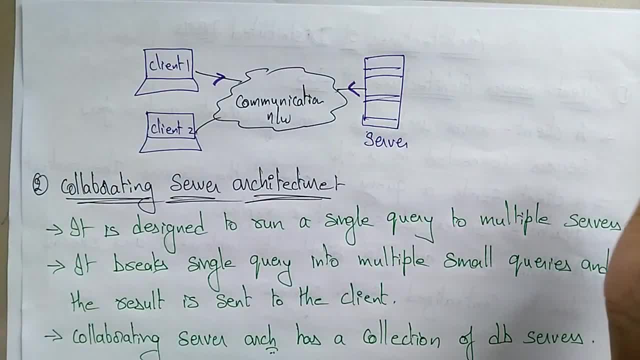 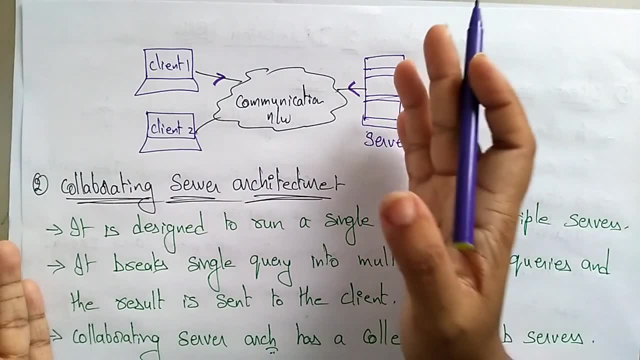 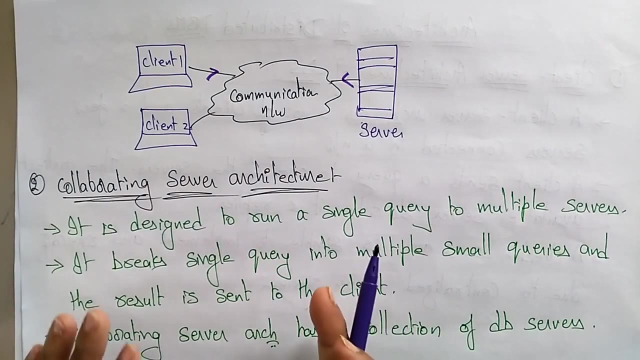 requesting. so many servers that are present over the network, the the most one it is depends upon the response of the server, which one is giving the fastest response that can communicate to that client and reply to the request. and the second type of this architecture of the distributed 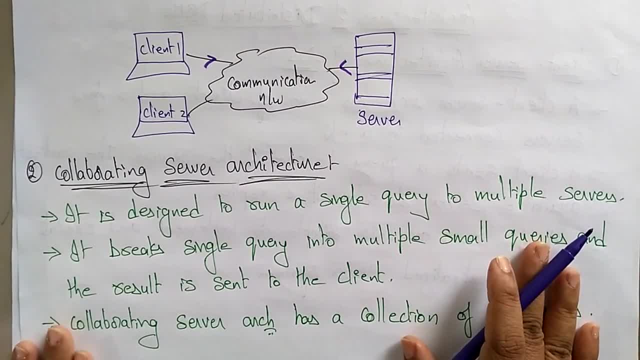 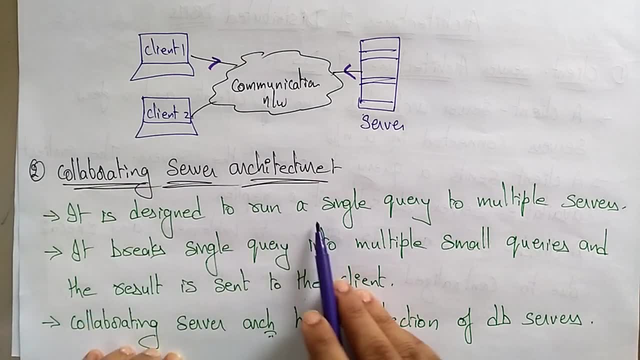 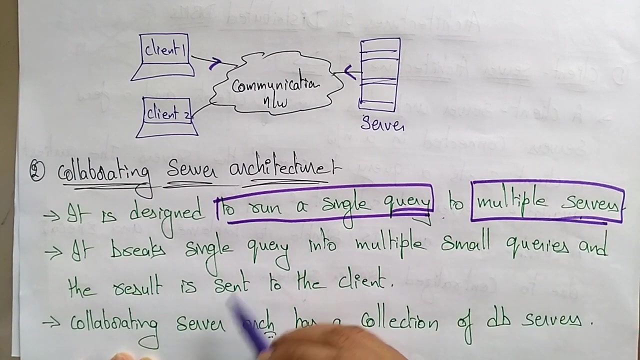 database management system is the collaborating server architecture. collaborating server architecture, so it is designed to run a single query to multiple servers. so the collaborating server architecture is designed in a way that to run a single query, to run a single query to multiple servers. it breaks single query into multiple small queries. 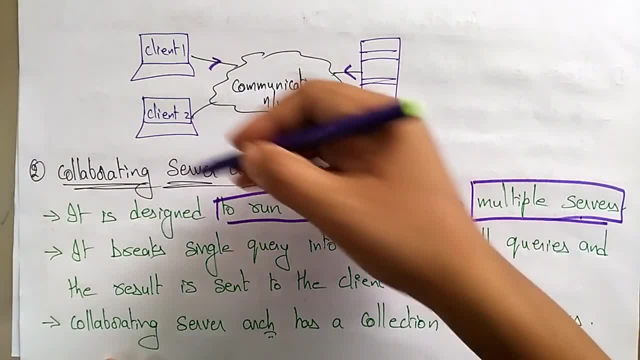 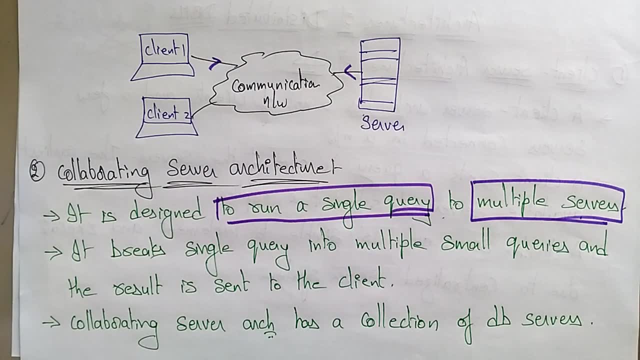 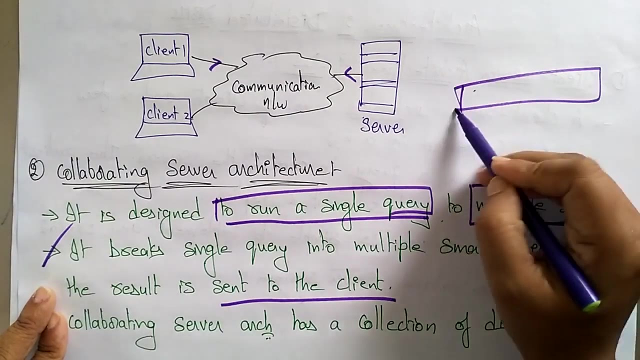 and the result is sent to the client. so see, here it's a collaborating means. each server is trying to solve a small task and all the tasks are collaborating and the result is sent to the client. that is, they are saying so it breaks a single query, a single query, into multiple. 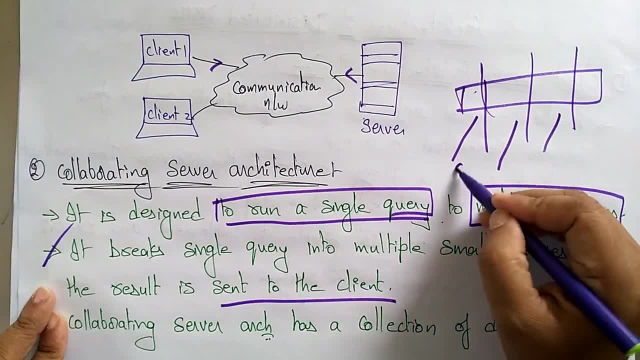 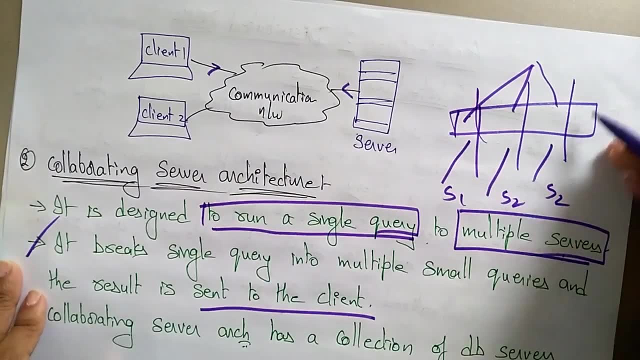 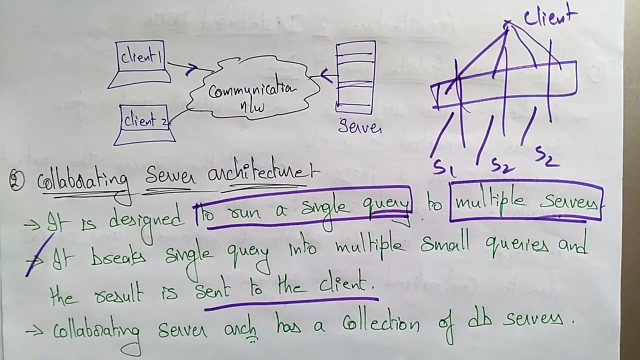 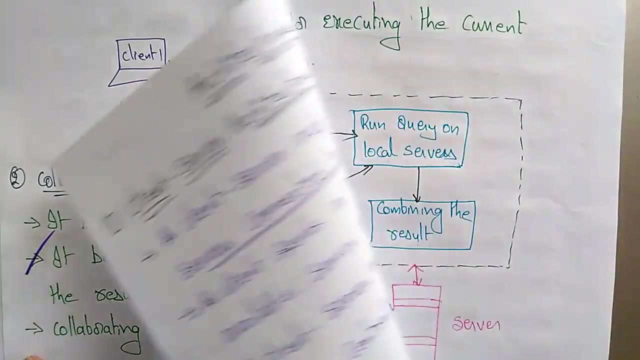 small queries and these small queries all sent to different servers. okay, after solving everything, all are collaborated and sends to the client and sent to the client. so this is a collaborating server architecture. here the collaborating server architecture has a collection of database servers. so see here this is a diagram of the collaborating sever architecture here. each 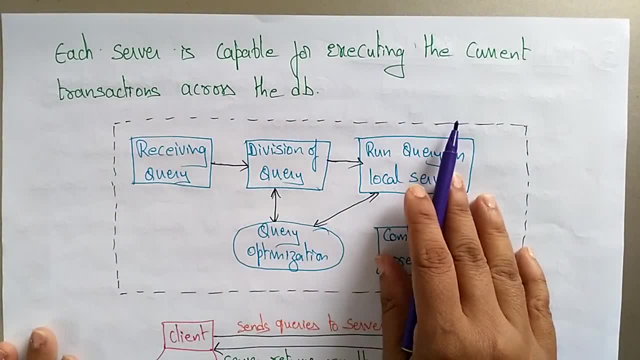 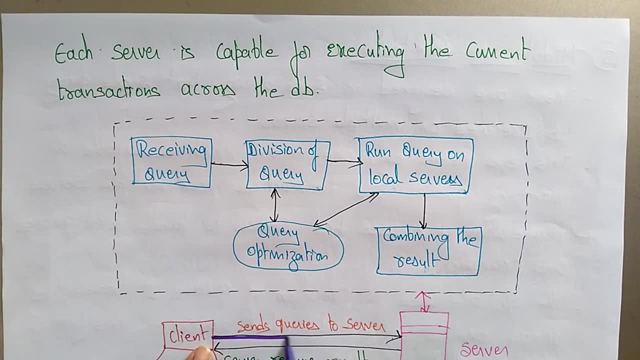 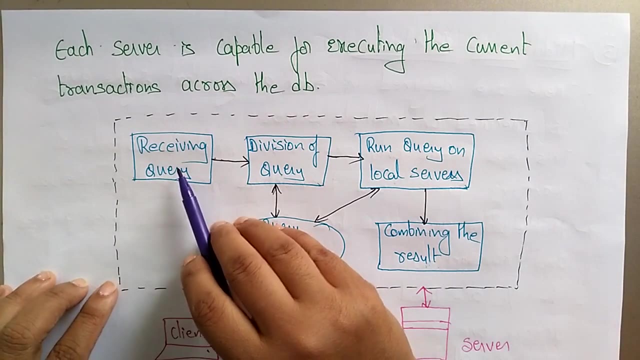 server is capable members executing the current transactions across the database. so the client is there, server is there. the client sends a query to server. the client sets a query to the server. so these server is going to do work, that Zurichie in the cavity. whenever it receives a query, the division of QUARgies, the query has to. 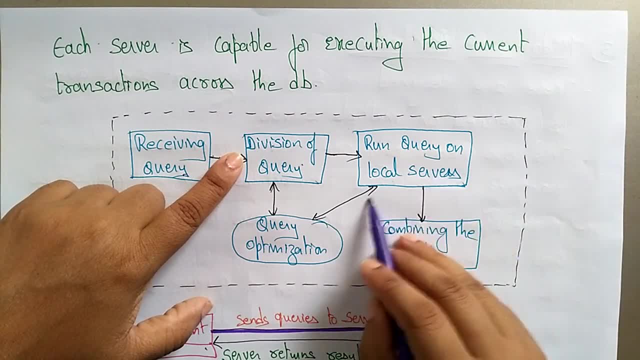 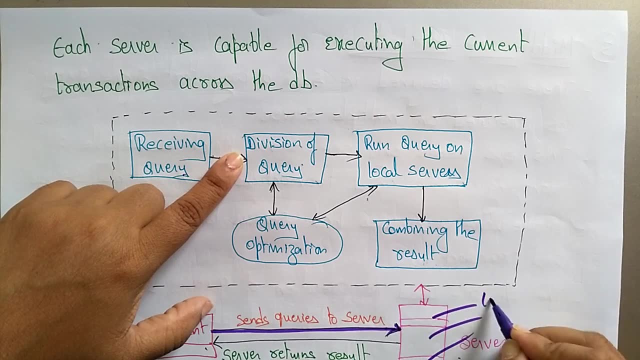 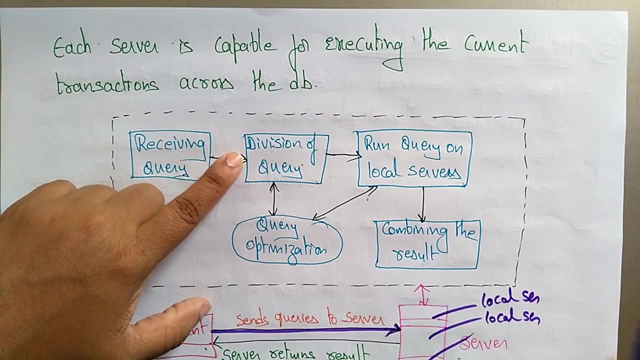 be wheeled down into a smallӠ small � pieces and run query on local servers in these servers they are having so many local servers okay so here so many local servers are present local servers local servers in a main server there are so many local servers are present so one query is taken from the client and division 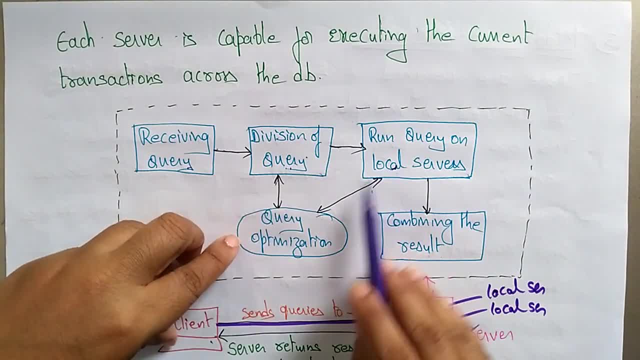 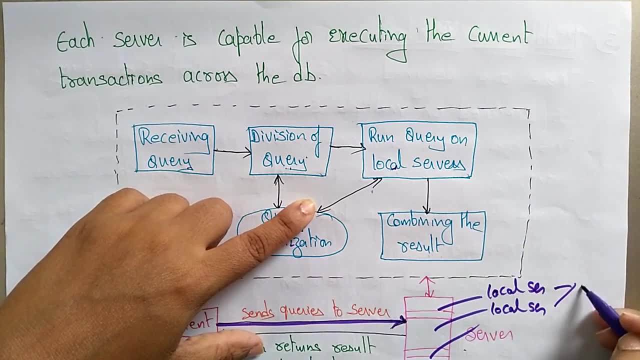 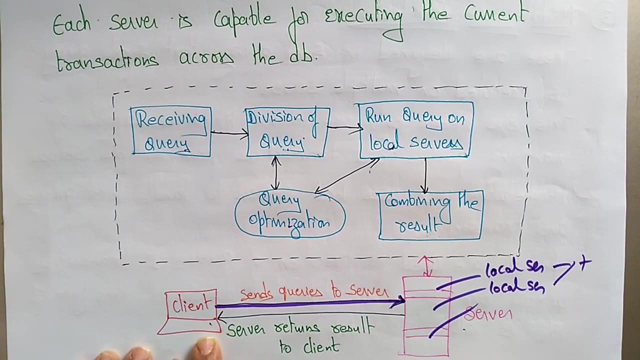 of that query and run on local query on servers. if any query optimization is there that checks and combining the result all local servers. after completing it, combines the result and again sends that results to the server. that server returns results to the client. this is a collaborating server architecture. the name itself is saying that it is going to combine, combine all the local. 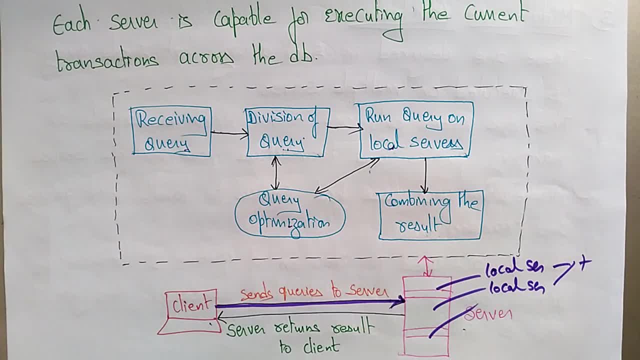 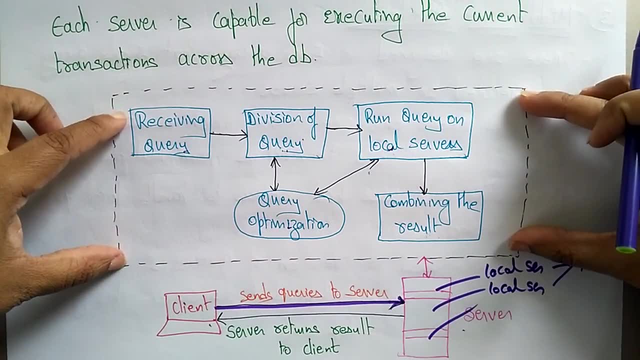 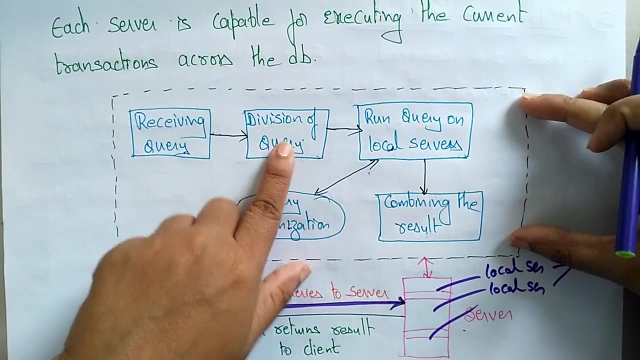 servers and send that results to the client. so here inside the server, what is going to be happen? this is going to be happen inside the server. this is going to be happen. so, receiving the query: after receiving the query, the division of query is taking place and run query on local servers. each division is 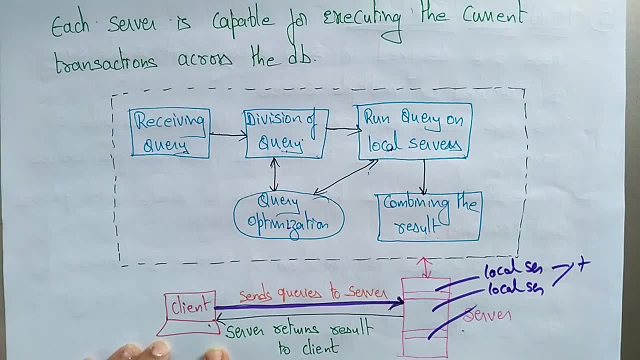 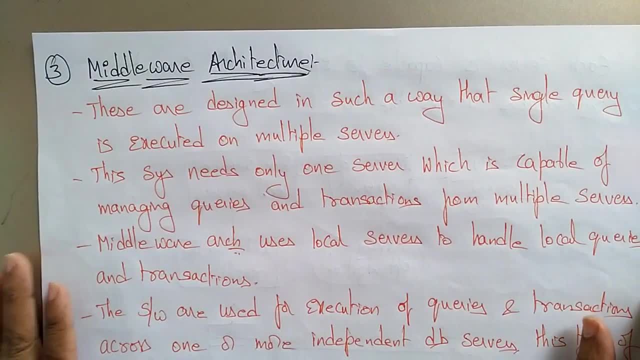 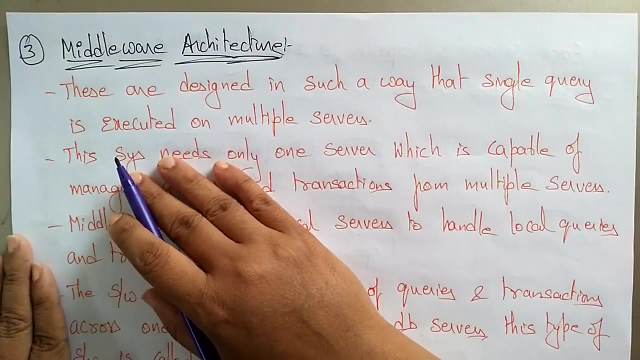 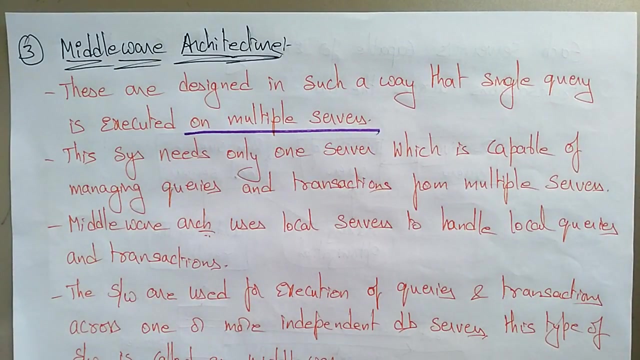 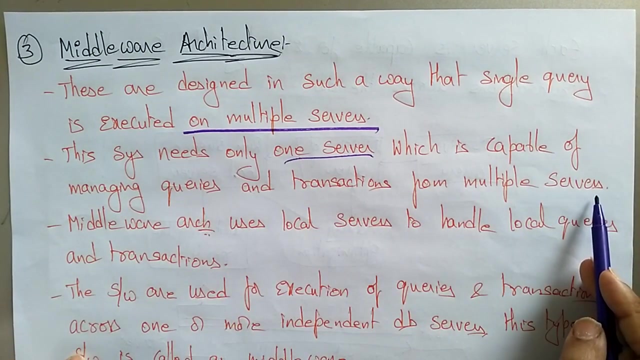 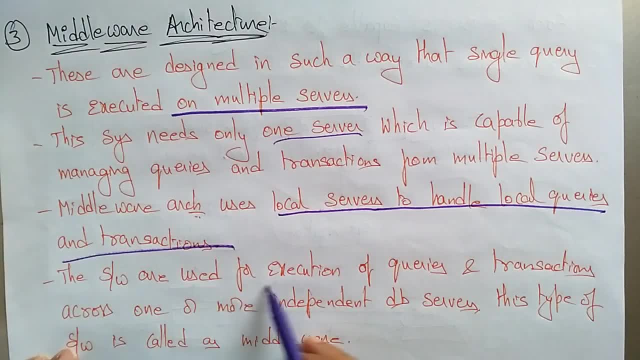 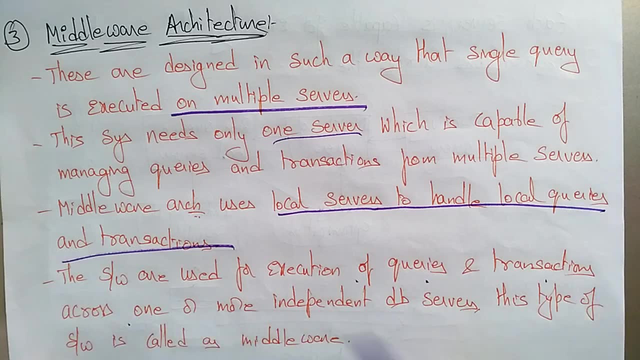 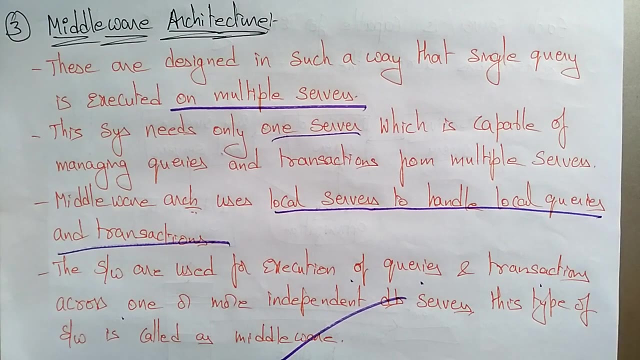